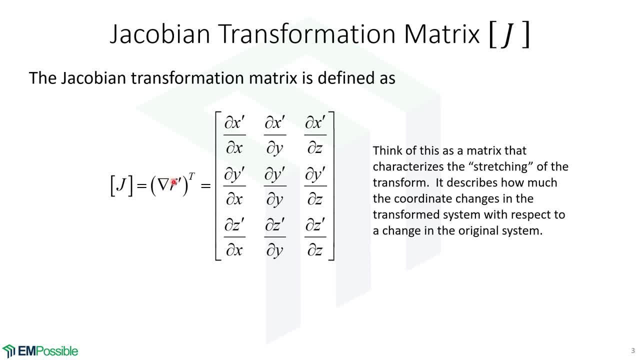 And then we transpose that, So the gradient of a vector. that's rather interesting. And it turns out the gradient of a vector is a tensor, And typically we're taught we can't have a gradient of a vector, But anyway we get this tensor. It's three by three, simply because we live in a three dimensional world. If we ever discover the fourth dimension, well, our Jacobian matrices will then be four by four, But right now they're three by three. 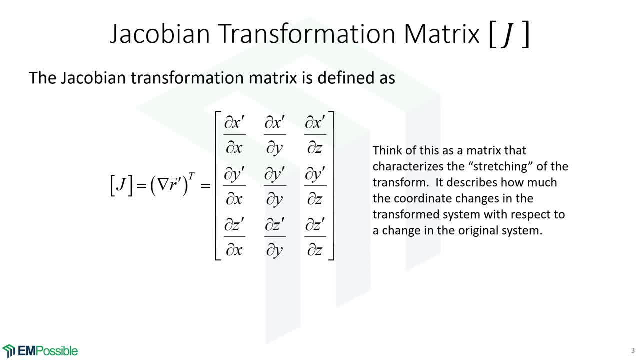 And we can think of the elements of this. The first thing to consider is sort of quantifying the stretching. So, for example, let's pick a few of these, Let's pick dx prime with respect to dx. So this means, if we move left and right in our original coordinate system, how far left and right in our transform system does that take us? And we look at the second term, the partial derivative of x. 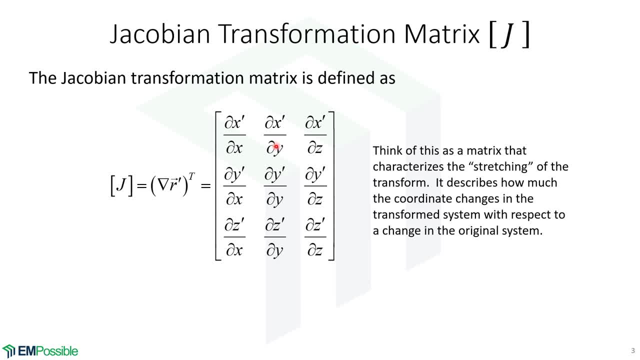 prime with respect to y, And so this means in our original coordinate system, if we're wiggling a little bit in the y direction, how much left and right does that take us in our transform system? And we'll do one more. 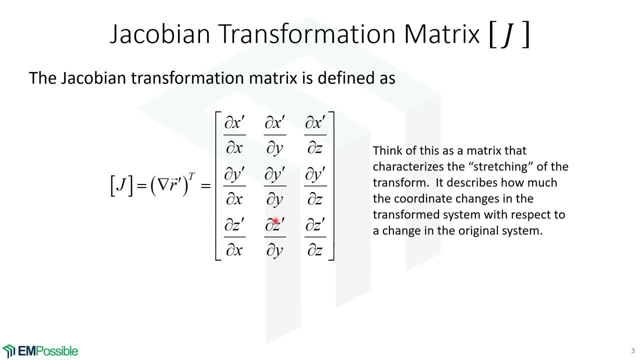 We'll look at this one. How about this? So the derivative of Z prime with respect to Y? So here, if we wiggle a little bit in the Y direction in our original coordinate system, how much does that take us in and out of the screen? 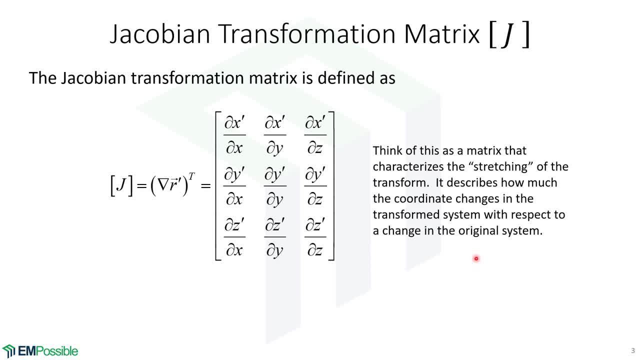 Boy, I can't really do that one, can I? Maybe I chose poorly, but you know how much in and out of the screen does that take us in the transform coordinate system. So that's how to think of this Jacobian transformation matrix. 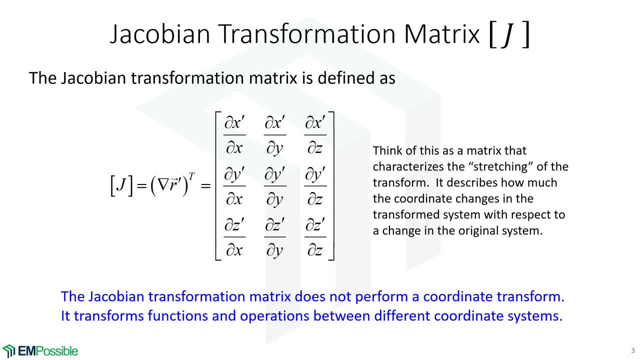 The other thing I'll mention is that the Jacobian matrix does not actually perform the coordinate transform That happened on the previous slide. Somehow we have functions that we can calculate our new coordinates from the old ones. This is something different that we use it. 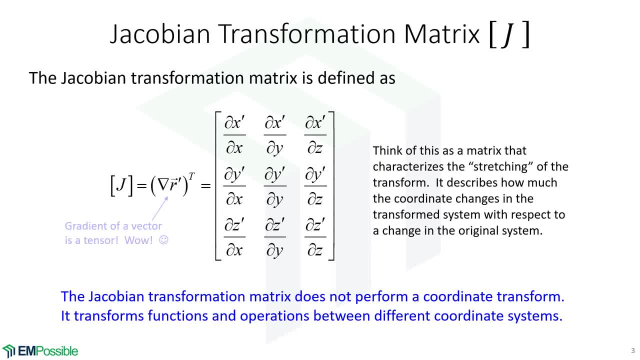 to do some different things that we'll get into. And the last thing I'll leave you with: that's sort of interesting that here we actually have the gradient of a vector that very often we're told can't happen, And it turns out it's a tensor. 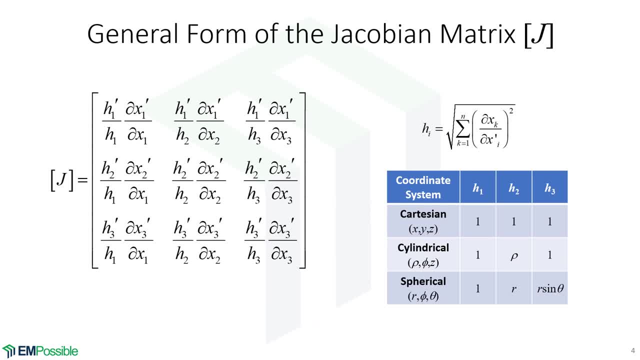 So I think that's pretty cool. There's a bit more general form of this Jacobian matrix that includes some scale factors, And what you'll see is that there's a scale factor associated with the numerator of our partial derivative and one associated with the denominator. 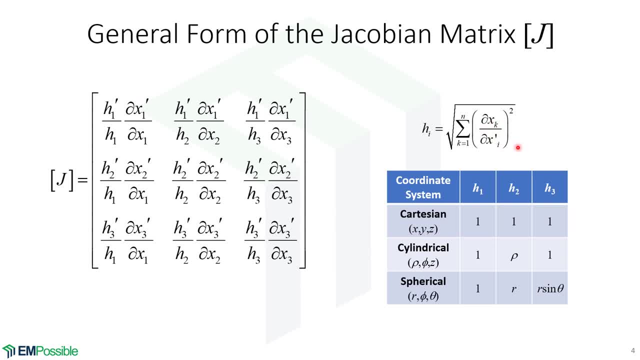 And we define that over here from our partial derivatives that are populating. So the Jacobian matrix, And what I've done is just summarize this for three different coordinate systems, the three that we most commonly use, And so for Cartesian, the scale constants are just one. 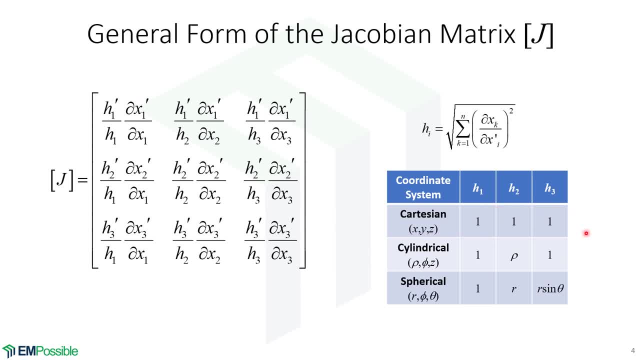 And so they're really not even there, And that's why we presented the Jacobian matrix that way the first time. But if we're ever writing this Jacobian matrix in different coordinate systems, like cylindrical, spherical, well, these scale factors come in. 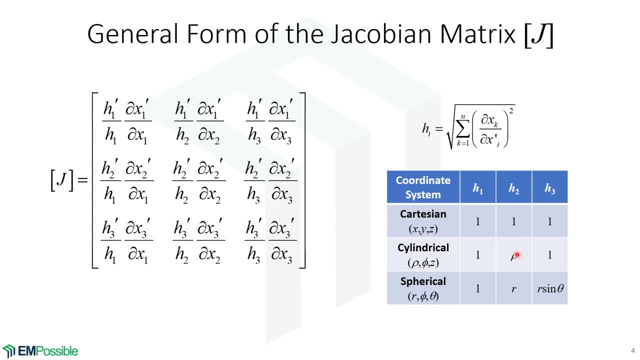 For example, our H2 is going to be a row, Our H2 will be a number, An R in spherical coordinates, An R sine for the H3 in spherical coordinates. So just keep this in mind And those scale factors. they're defined this way. 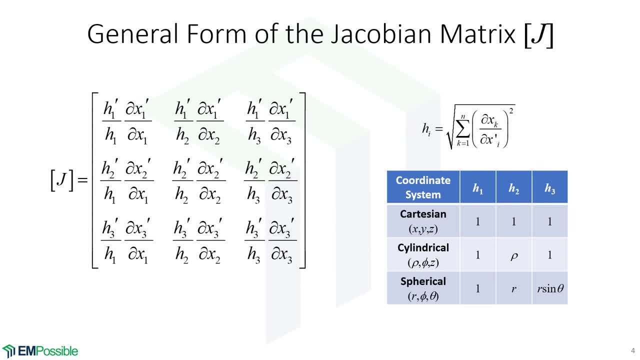 Most of the time we're working in Cartesian coordinates. Well, I should say, most of the time when we jump to our numerical solution, we're working in Cartesian coordinates and we don't have these because they're all just equal to one. But, for example, cloaking the big famous Duke cloak. 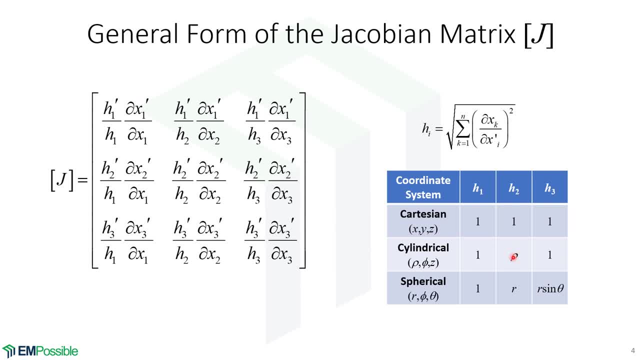 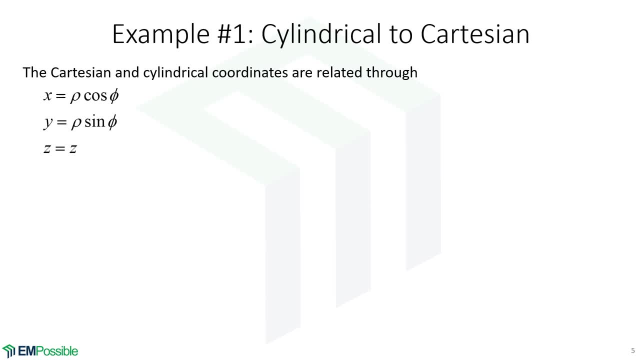 well, that was in cylindrical coordinates And there is a row here And for H2, and so we do need to consider those scale factors. So this is the most general form. Let's have some examples of calculating a Jacobian matrix. 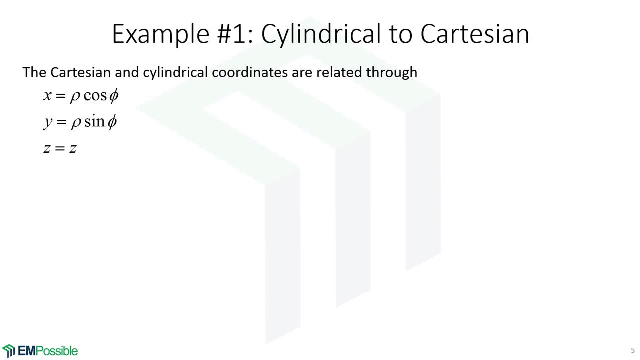 Let's say we just would like to convert from cylindrical to Cartesian coordinates. So we're going from cylindrical to Cartesian, So we need some equations to do that. So we're going to Cartesian, So we need to calculate X, Y and Z as a function. 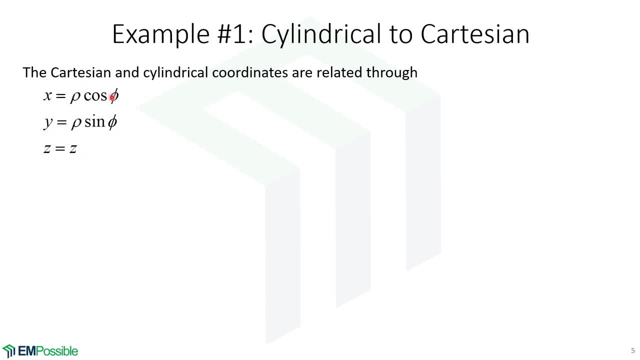 of our cylindrical coordinate parameters, which are rho, phi and Z. Well, the easy one, okay, Z equals Z. That's an easy one, And this should be pretty familiar of how we calculate X and Y from rho and phi in cylindrical coordinates. 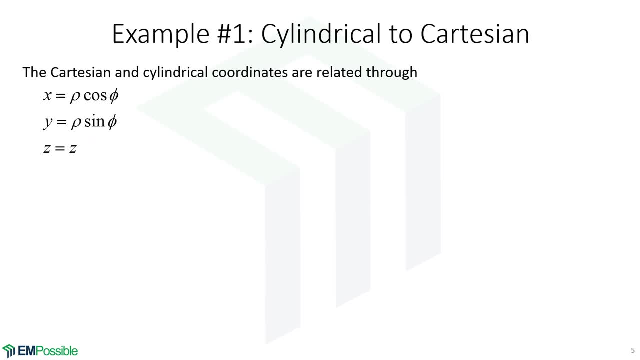 So what would the Jacobian be for this transformation matrix? So here's how we would define our Jacobian, And now what we want to do is go one term at a time and calculate those partial derivatives. So our first one partial derivative of X with respect to rho. 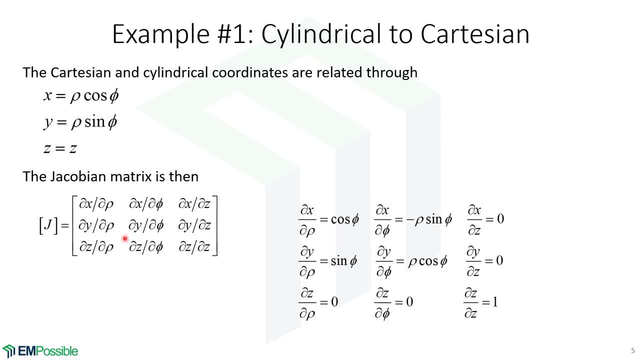 Oh, I'll mention one thing. Notice, there's no scale factors here, and that's because we're in Cartesian coordinates. Anyway, back to this dx, d, rho. So we want to take the partial derivative of X with respect to rho. 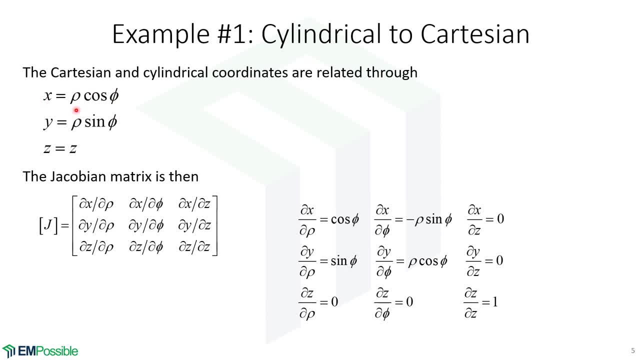 So that means we go up to this equation and take the partial derivative of it with respect to rho. Well, that's just going to be cosine phi. and there we have cosine phi. So now the partial derivative of x with respect to phi, and that's a. 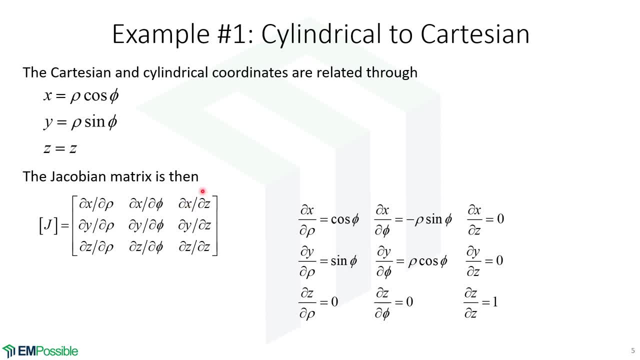 negative sine phi. Now we have our third term, partial derivative of x with respect to z. Well, there is no z in this equation, so in fact that term in the Jacobian is zero: dy d rho. Now we're at the second equation, and so we're going to be taking the partial derivative of this with respect. 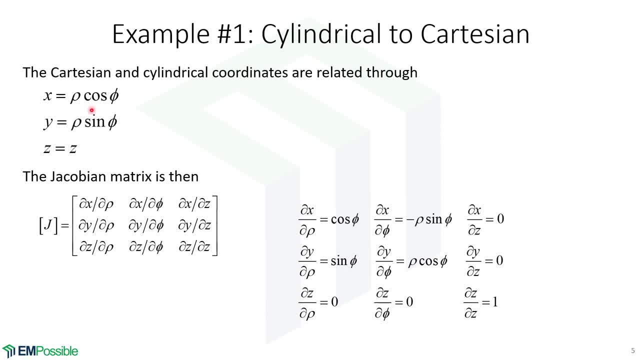 to rho, then phi, then z. So with respect to rho we just end up with sine phi. With respect to phi, that's a rho cosine phi- and with respect to z, there is no z here at the constant, so the partial derivative is zero. And then finally the partial derivative of z with respect to rho, phi and z. 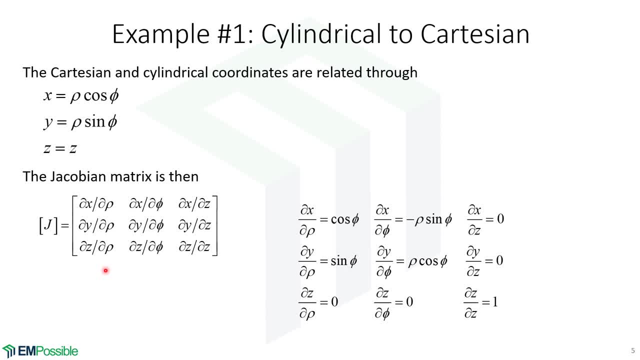 Well, we have a simple equation: or z equals z, So the partial derivatives with respect to rho and phi. there is no rho and phi, So that's zero, And then, of course, the partial derivative with respect to z, and that's just one. So we can throw all that back into our Jacobian matrix and this would 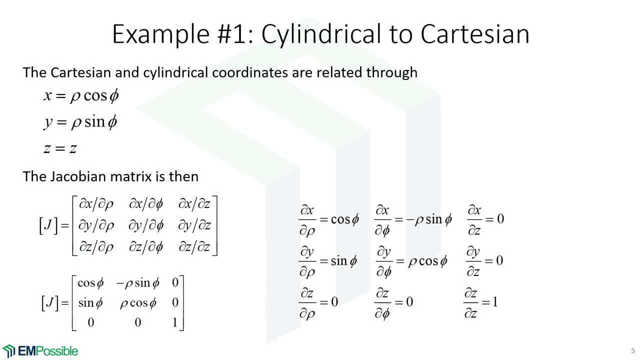 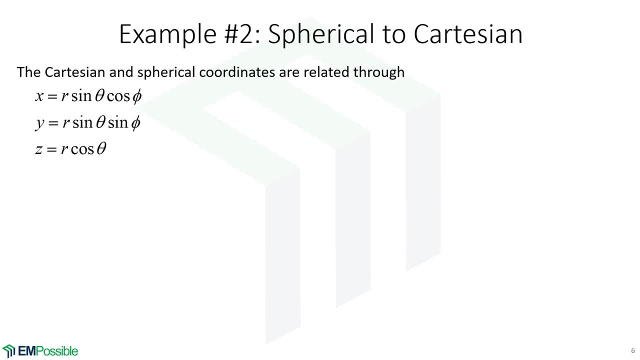 be the Jacobian matrix for cylindrical to Cartesian. A second example: How about spherical to Cartesian? So the first thing is we need our equations to do the coordinate transform. So we need x y z with respect to z. So we need x y z with respect to z. So we need x y z with respect to z. 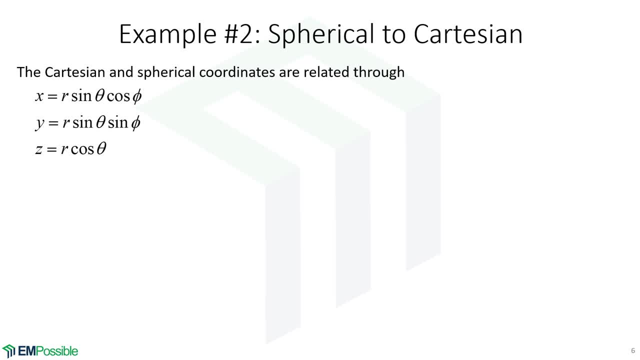 So we need x, y, z with respect to our spherical coordinates. and these are the three equations and that should be familiar to you. Next thing, we define our Jacobian Notice again: no scale factors, right, because we're in x, y, z, These are Cartesian coordinates, so all those scale factors are one. 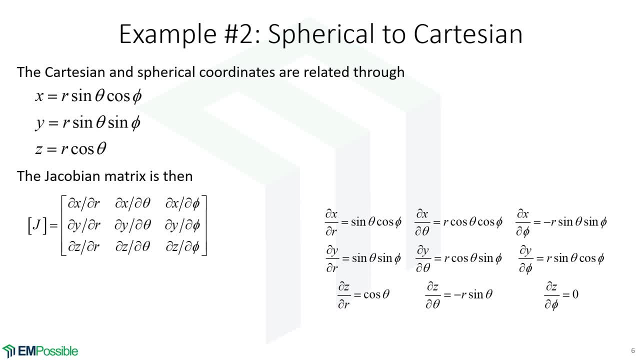 and we go one at a time. So our first element is the derivative x with respect to r. So that's this first equation. and so well, r is just out here. so it's just simply: sine theta cosine phi. This is a constant multiplying r. That's our first element. Now we need the partial. 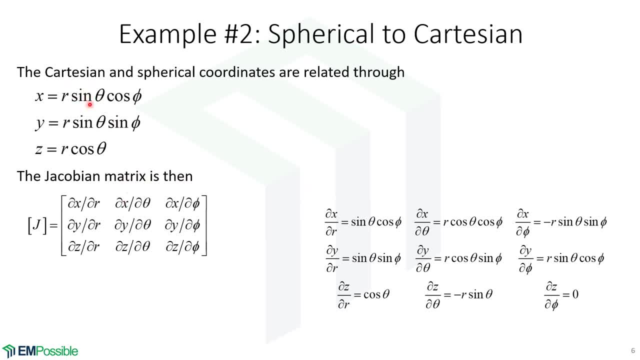 derivative x with respect to theta. Well, now we actually have a sine theta. It's a little bit more complicated, and so the derivative of sine theta is cosine theta. So we end up with an r- cosine theta, cosine phi- Now the derivative x with respect to phi, and we have a cosine phi, The derivative. 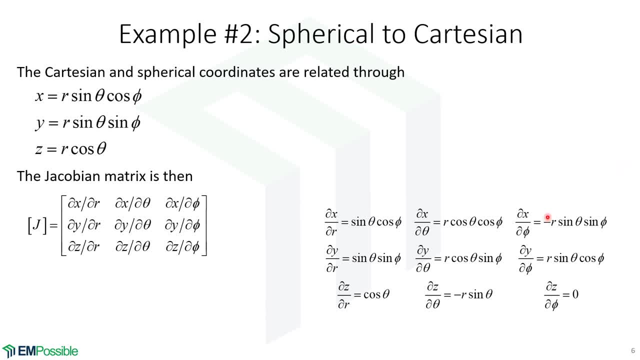 cosine phi is negative sine phi, So we have a negative r sine phi. Next line Now we're taking the partial derivative y with respect to r, then theta, then phi. So here's our equation. for y, The partial derivative with respect to r is simply just. 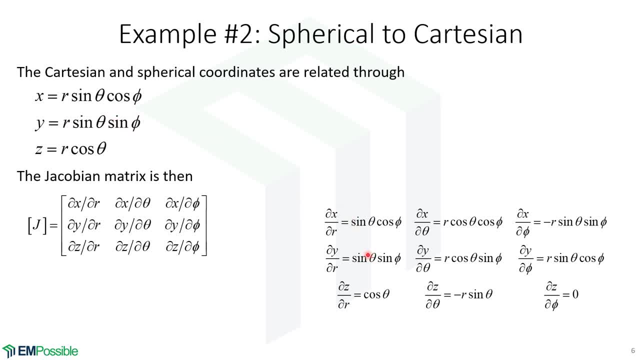 sine theta, sine phi. That's our first element here. Then, with respect to theta, well, the derivative sine theta is cosine theta, So we have r cosine theta, sine phi. And then, with respect to phi, derivative of sine phi is just cosine phi, So we have r sine theta, cosine phi. Last line, Our z equals r cosine theta, and we want the partial. 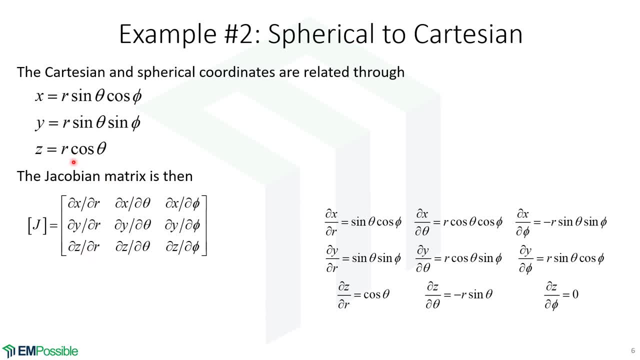 derivative of that with respect to r, then theta, then phi. Partial derivative with respect to r is just cosine theta, Partial derivative with respect to cosine theta. Well, the derivative of cosine is negative sine. So we have negative r sine theta, And then partial derivative with respect to phi. 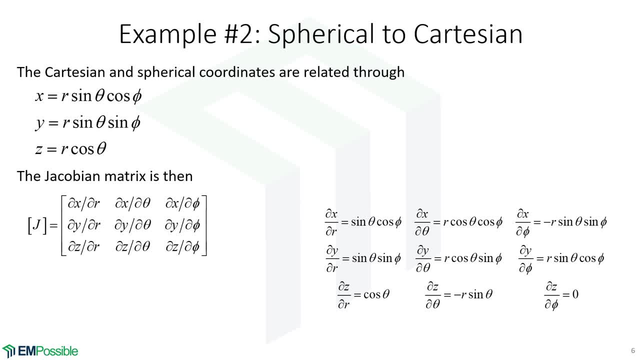 There is no phi up here, so the partial derivative is zero and we can throw that back into the jacobian. so this is the jacobian for the transform for spherical to cartesian, and that's really it. now the algebra and taking these derivatives might get a little bit complicated for certain transforms, but it's really a straightforward. 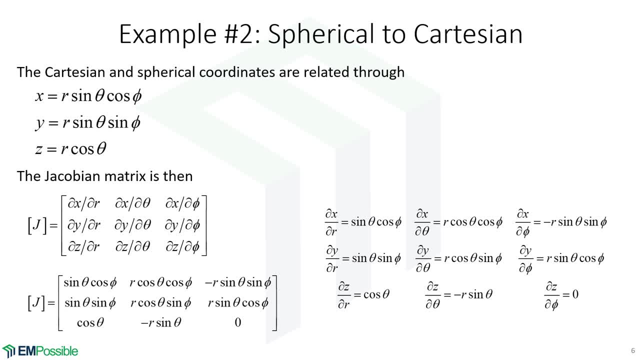 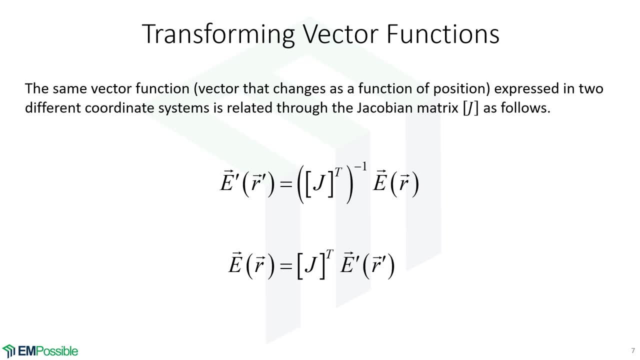 process to construct this jacobian. okay, we have the jacobian. we can now use this to transform vector functions and we have these in Maxwell's equations. right, our electric and magnetic fields are vector functions. so if we want our electric field in our transform coordinate system, that 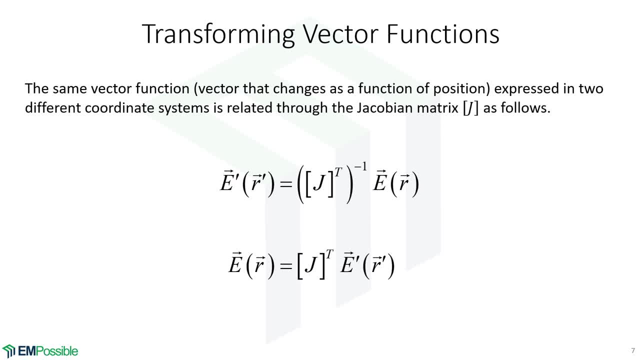 we're indicating with the little prime notation there. well, we pre-divide by the transpose of the jacobian, so jacobian transpose inverse times e will give us the transformed e, and we can do it the other way around if we have the transformed e simply pre-multiplied. 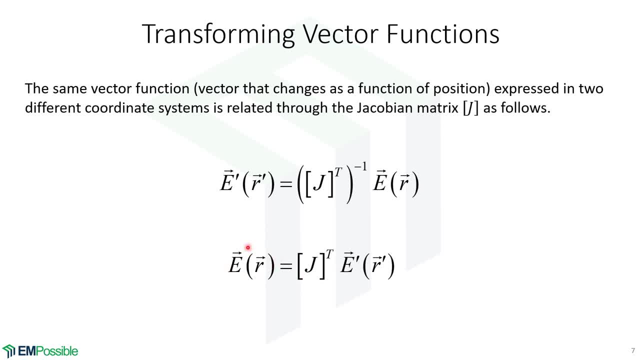 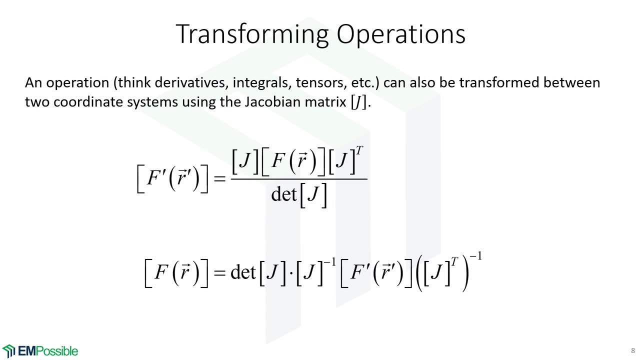 that, by the transpose of the jacobian, gives us the field in the original coordinate system. so that's one use of the jacobian transform vector functions. well, we have other things in Maxwell's equations, we have our operations. these are all the things happening to those vector functions. so operations think things. 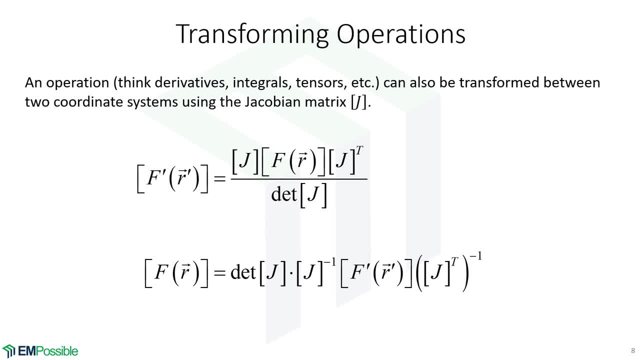 like derivatives, integrals, and our tensors, our material properties, our mu and i, epsilon, and maybe we're thinking: well, why aren't those functions? well, yes, they're functions to us, but in terms of the differential equation, those are operations happening on to the field quantities. they're point by point multiplications that are happening. 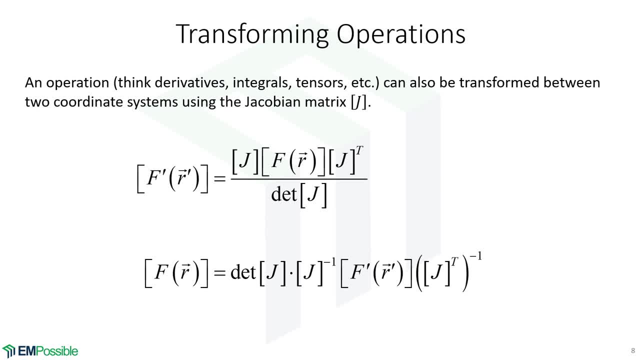 so those truly are operations, and this is how we transform operations using the jacobian, no matter what that operation is. so let's say we have some operation f well, we're going to pre-multiply by the jacobian post, multiply by the transpose of the jacobian and divide by the determinant of the. 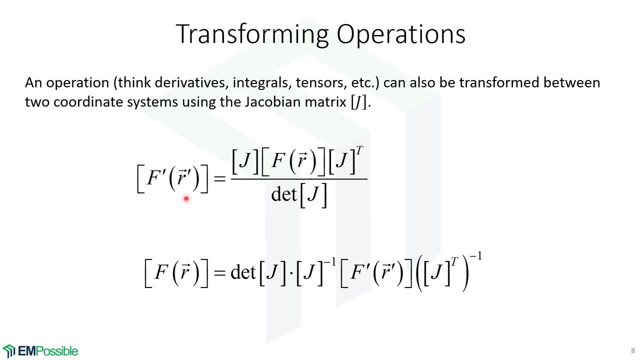 jacobian. that gives us that same operation in our transform coordinate system. now we can simply solve one for the other. we can reverse this and we can write our original operation as the operation in the transform coordinate system. now we're pre-dividing by the jacobian. 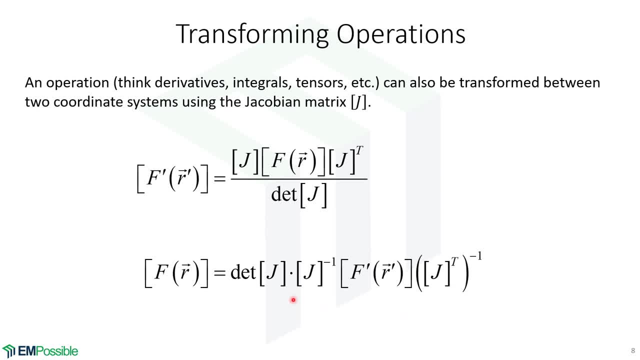 we're post dividing by the transverse of the jacobian, and then we're also multiplying all that by the determinant of the jacobian, and so we can use the jacobian to go either way. so that's the purpose of the jacobian: it makes. it makes transforming our operations. and 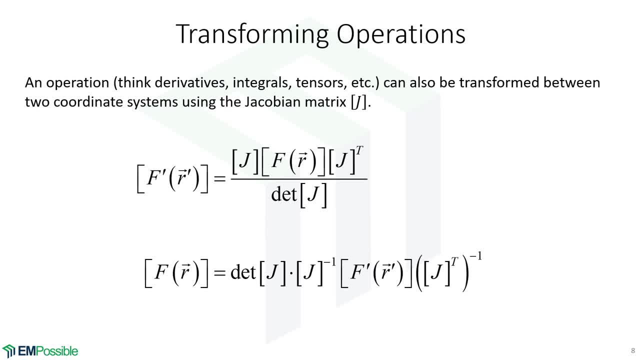 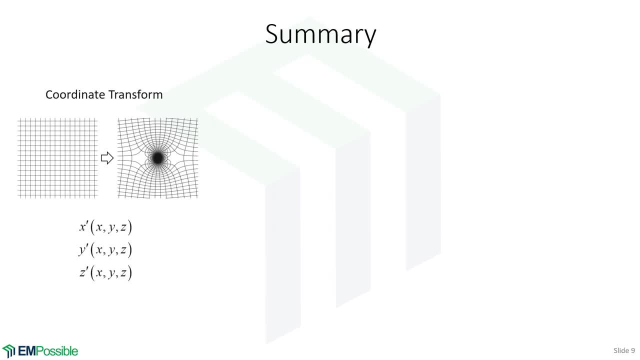 our vector functions quite easy. so here's a summary of what we've done in this video. we started with a coordinate transform and- and this actually, a lot of times, is the hardest part of the jacobian process, because we're going to be using a lot of equations that do this transform.